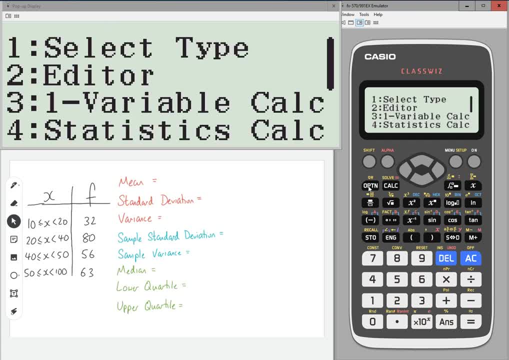 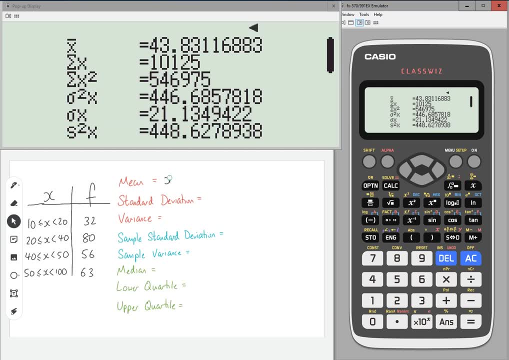 That's why we're using the midpoints. So once you've done that, press option number three, one variable calculation, And here we go. So the mean is X bar, which is 43.83116883.. Below that is the sum of X and the sum of X squared, which is useful, but not what we're looking for today. 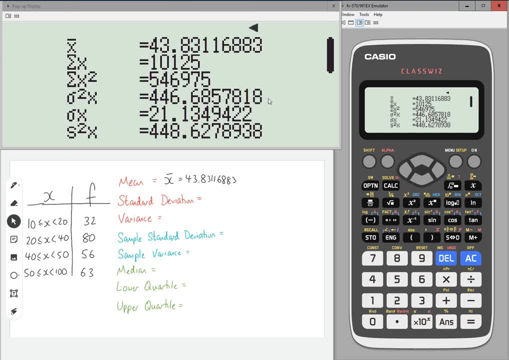 Sigma squared is the variance. So sigma squared is 446.6857818.. For those doing OCD, For those doing OCR, MEI, this is the mean square deviation Below, that is sigma X, which is the standard deviation, which is 21.1349422.. 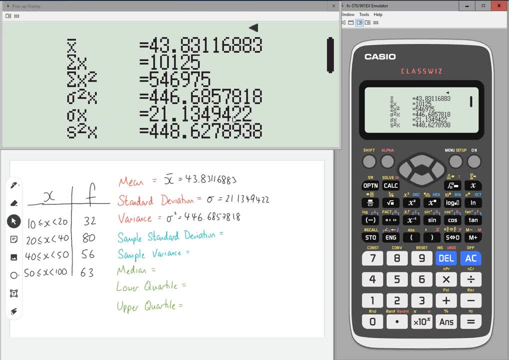 So for MEI this is the root mean square deviation. Below that is S squared, which is the sample variance, So 448.. Oh, sorry, I'll just put the S squared there as well, for consistency: 448.6278938.. 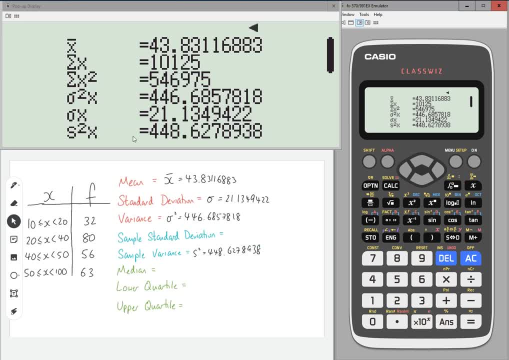 OK, So for MEI they would just refer that as the variance, But for the rest of us that's the sample variance. They may also refer it as the sample variance And then SX, the sample standard deviation. This is 21.18083789.. 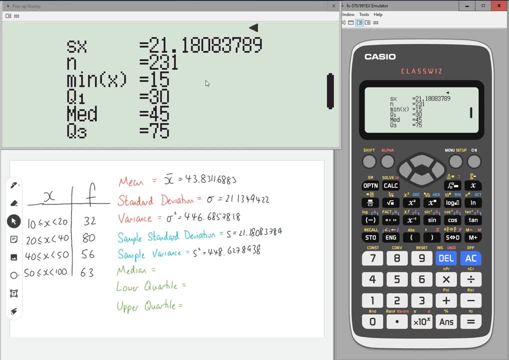 OK, Now what's important is that below this, where it goes into the median and quartiles, this is nonsense. OK, Now, the reason why you cannot use this information is because we've typed in the data as if there were 3215.. 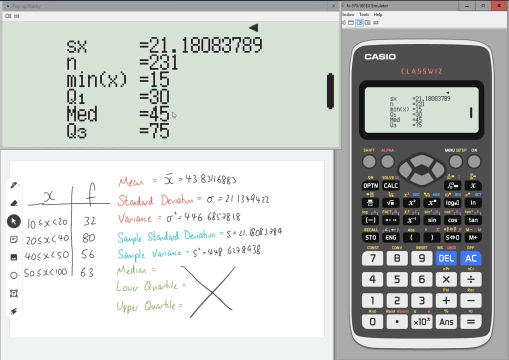 Okay, that there were 80 30s, there were 56, 45s and 63 75s. that is how it is calculated: the median and quartiles. it is not taken into account that this data is grouped frequency, and so, in order to work,